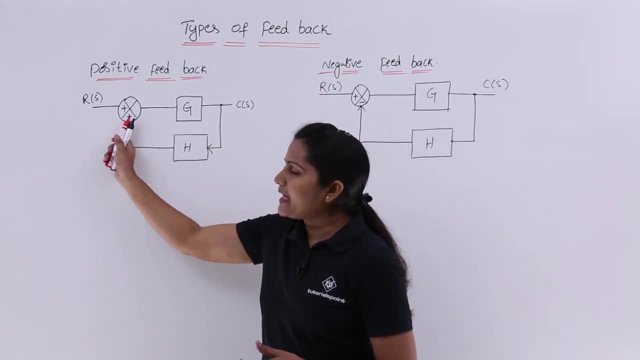 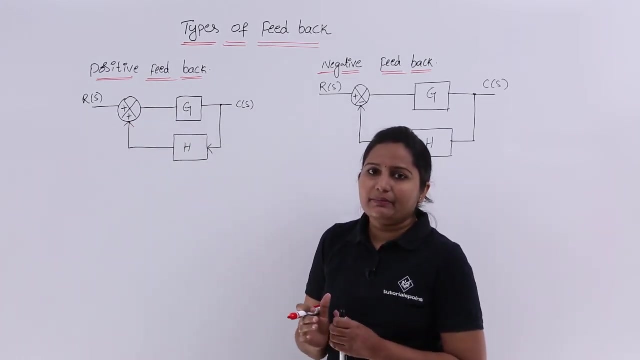 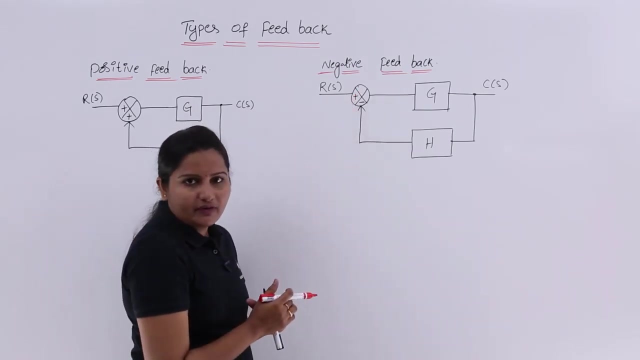 r of s here and here. whatever feedback is there that we are adding here. Here you can observe a positive or addition symbol. So here we are adding the feedback, So we are call, we are going to call this Feedback as positive feedback. Similarly, coming to this feedback, we are subtracting that feedback. 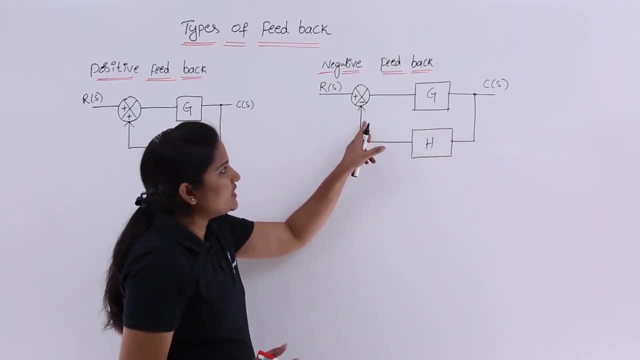 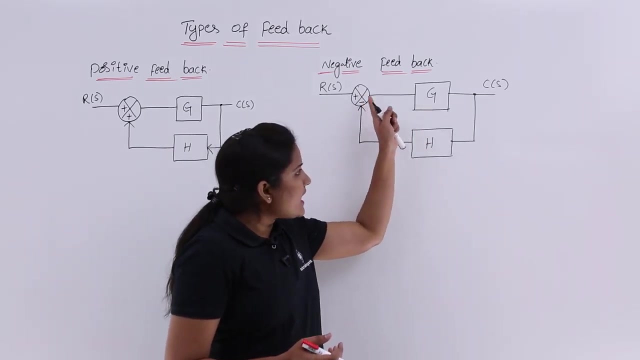 element. That means so here, c of s into h. we are going to subtract here. So from r of s, we are going to subtract c of s into h. So this type of feedback is called as negative feedback Generally in this side, the feedback side. if you saw negative symbol, that is called as negative. 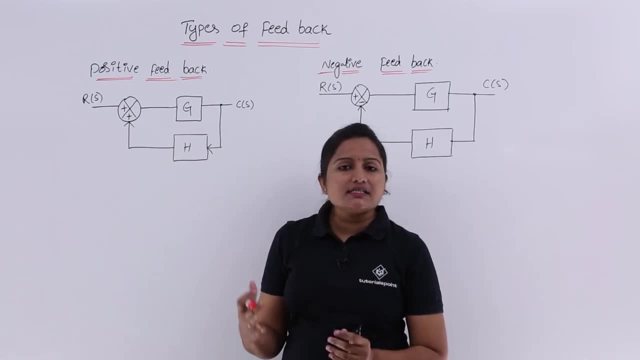 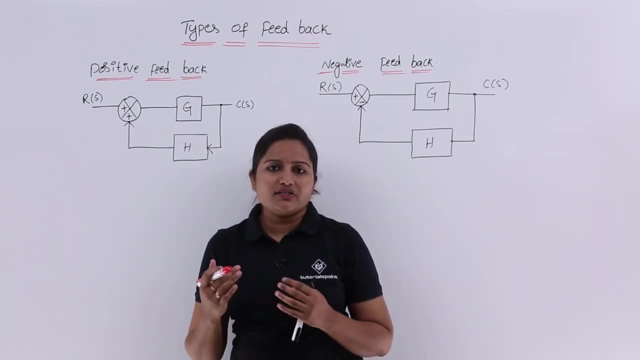 feedback. If you saw positive or plus symbol, then that is said to be a positive feedback. Then, coming to the transfer function of these two systems. So we know that the transfer function is the ratio of output transform by input transform. Here we are having output. 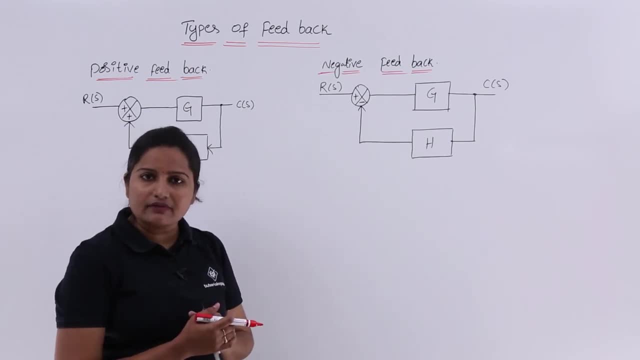 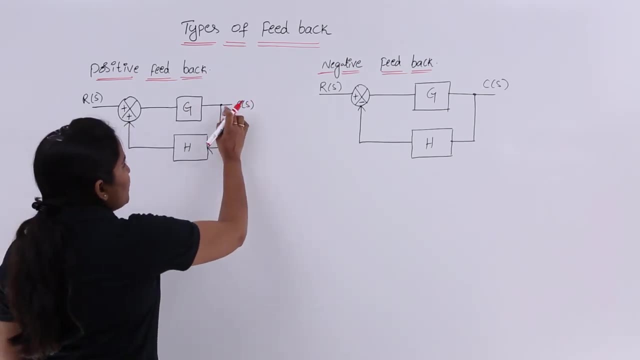 transform as c of s and input transform as r of s in both positive and negative feedback systems. So here I am writing like this. So this side, this point, at this point you are having c of s. This c of s is multiplied with this feedback gain: h. 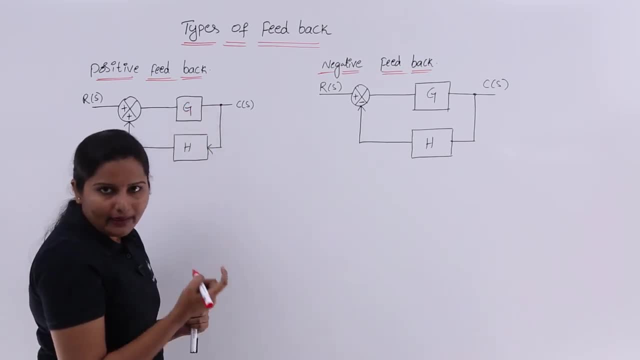 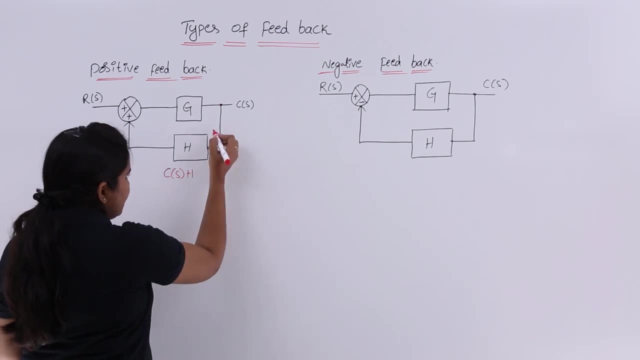 where h is the feedback gain and g is the open loop gain of the control system. So the value here is c of s into h. The value here in this line is c of s into h. This signal is multiplied with this gain. Now I am going to add this r of s with c of s into h. 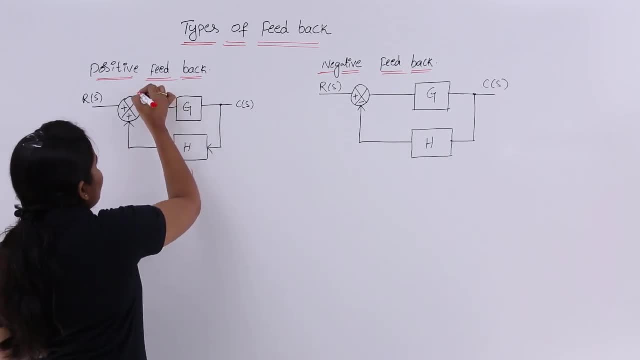 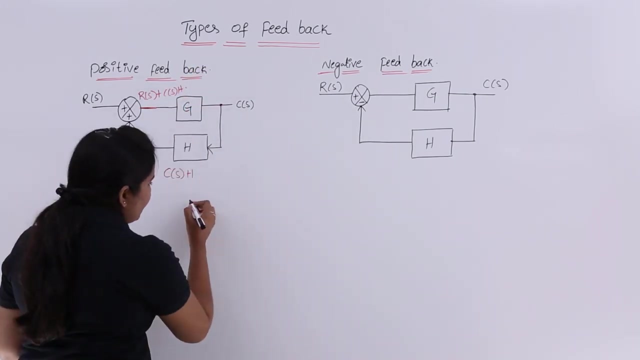 So the resultant value from this line is equivalent to r of s plus c of s into h. Now if you want to write this c of s equation after giving this feedback, then that equation will be: c of s is equivalent to this r of s. 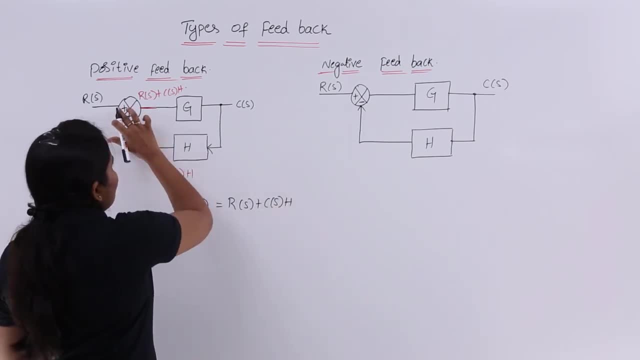 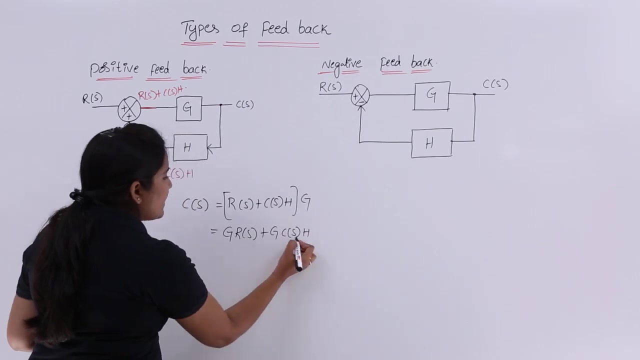 plus c of s into h. This is the signal out from here, and the gain is into g. The gain is g. So now this is equivalent to g into r of s plus g into c, of s into h. We are having c of s here, and here I am sending from right to left, So 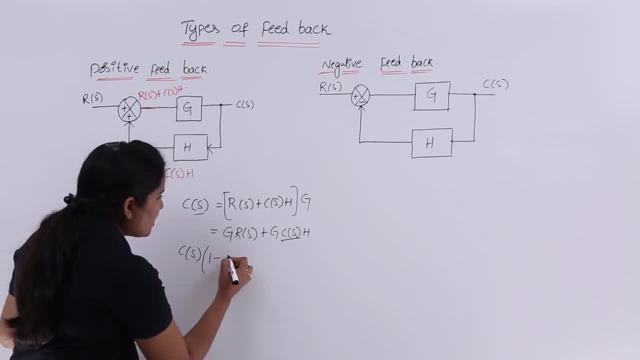 I am taking common of this c of s, I am going to get 1 minus g h is equivalent to g into r of s. As transfer function is equivalent to output. transform by input. transform c of s by r of s, then this is equivalent to g by 1 minus g h. This will be transfer function of positive. 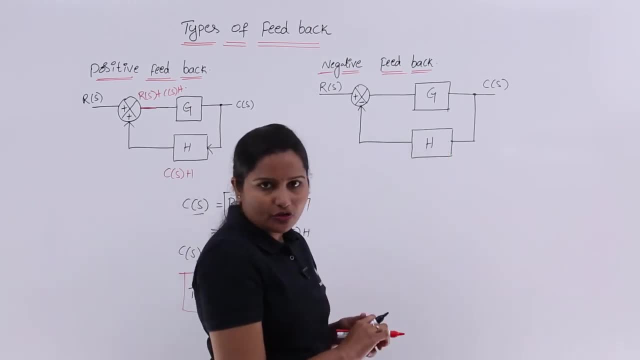 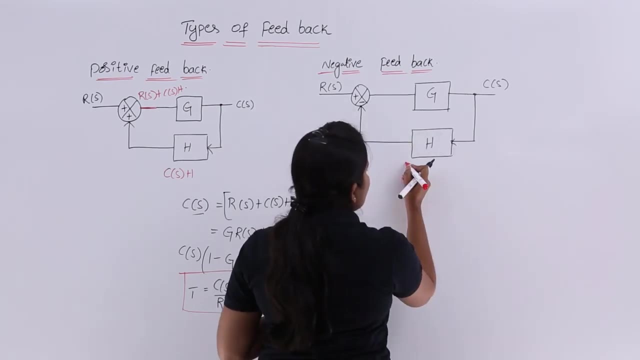 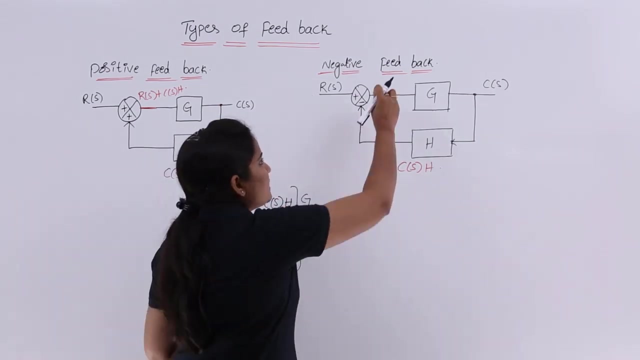 feedback control system, Coming to negative feedback control system. here also the value of this line. the value of this line is equivalent to c of s into h, but we are subtracting this value from the reference signal r of s, So the resultant value here the resultant. 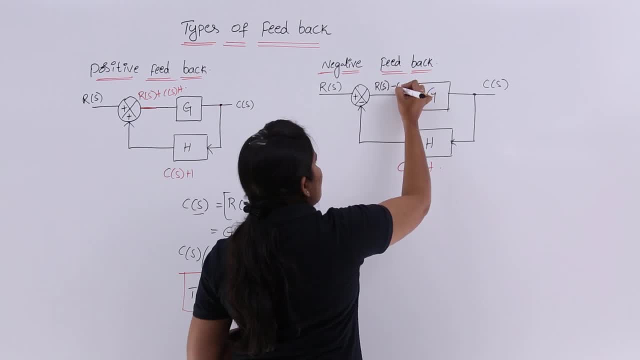 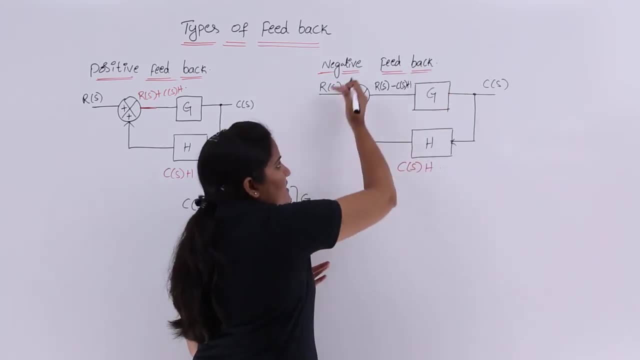 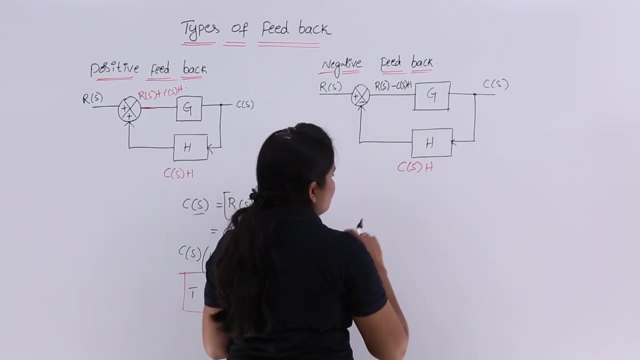 signal here is equivalent to r of s minus c of s into h, So the total line value will be: is equivalent to c of s. So, after giving this feedback, after getting this value, what is the value of c of s now means? c of s is equivalent to r of s minus c of s into h, into. 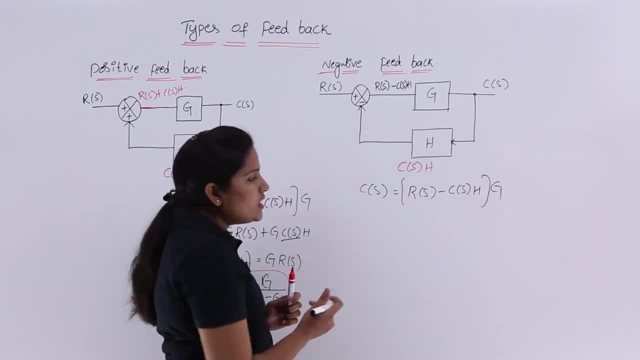 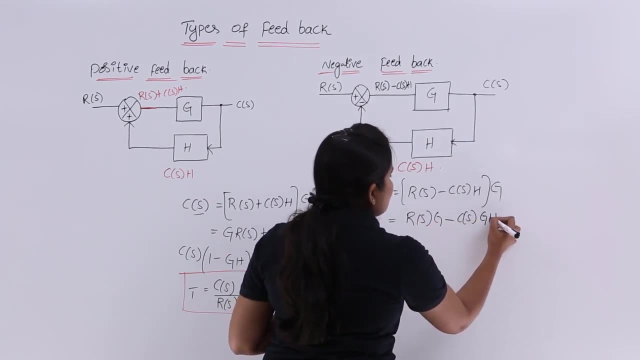 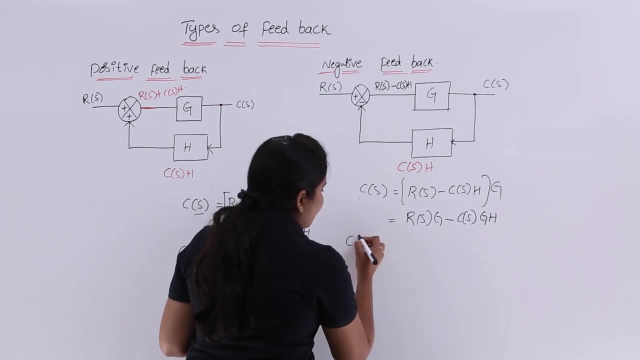 g. we need to multiply that gain this time. So this is equivalent to r of s into g, minus c of s into g h. So we are having c of s this side. also I am sending total c of s left side, So I am taking common of this c of s. I am going to get 1 plus g, h is equivalent. 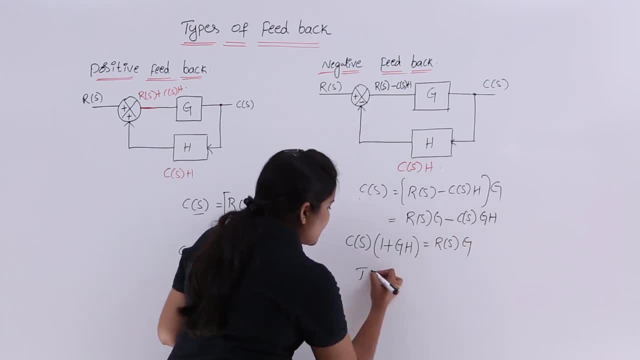 to r of s into g, As we know that the transfer function is the ratio of g. So output transform by input transform. our output transform is c of s. I am sending this r of s to this side, So I am going to get g by 1 plus g h. you just send this side, So